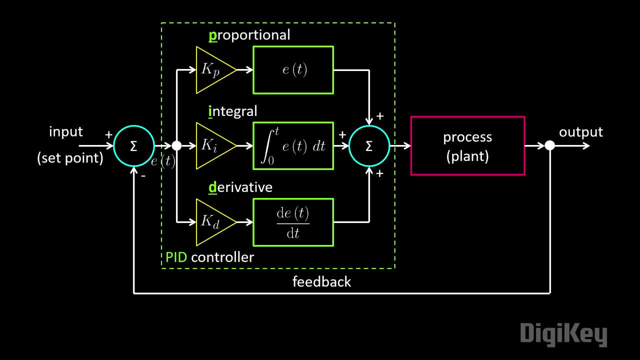 process or machinery. Don't worry about understanding this diagram quite yet. We'll work our way up to it throughout this video, But know that PID controllers are one of the most popular control theory mechanisms. If you're not familiar with it: control theory. 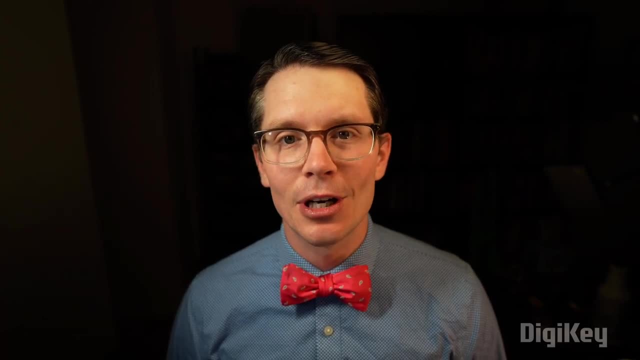 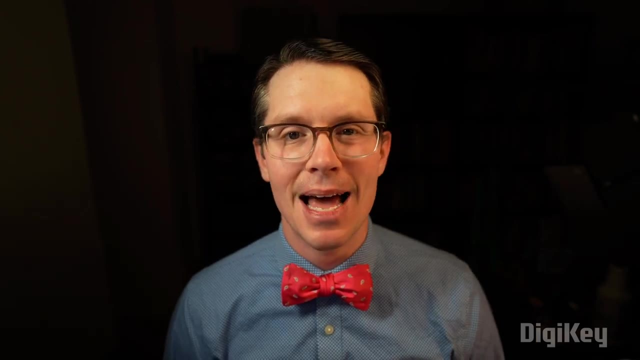 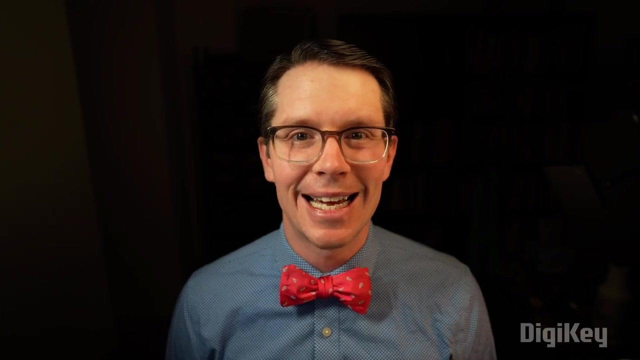 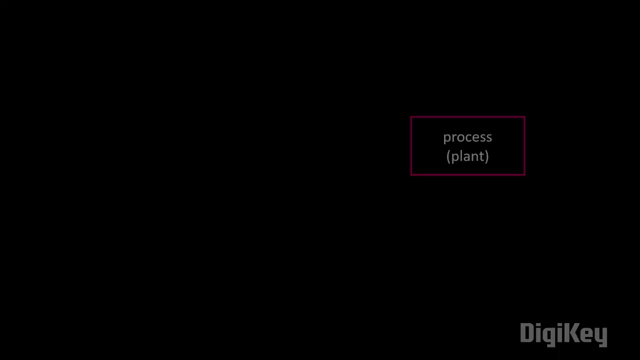 is a field of engineering and mathematics dealing with the control of dynamic systems. Often, these systems are mechanical and can be described entirely by math equations. I'll give you an overview of how PID controllers work and some examples of them in everyday use. Let's 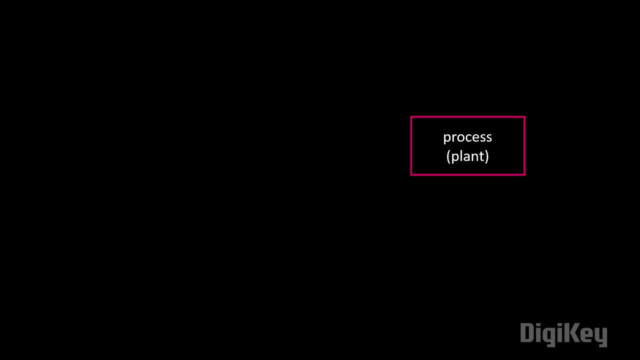 start with our system or subsystem that we want to control. This can be any process, piece of machinery, actuator or what have you. In control theory, you'll often see this referred to as a plant, which is a term that comes from the industrial revolution in the late 1700s. 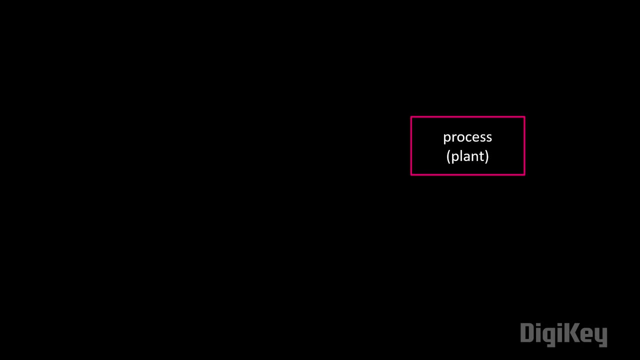 to mean something that has been planted in the ground for industrial purposes, such as machinery or tools. The process receives some sort of input signal and the output can be ideally measured. While controllers are extremely popular in the industrial world, they're not popular in industrial settings. Let's start with a more common example. Most cars have an accelerator. 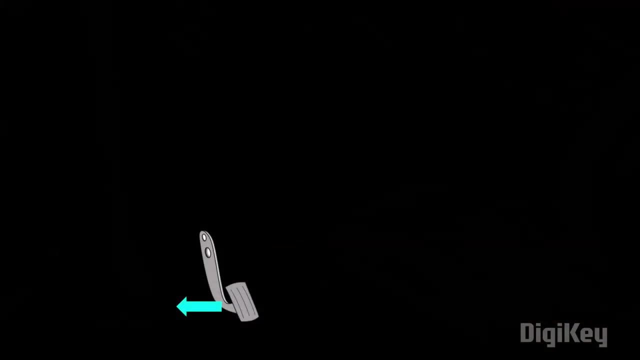 also known as a gas pedal. When you press the gas pedal, the car responds by allowing more air and fuel into the engine. As a result, your engine produces more power, which increases your speed. Now most accelerators are not binary. You can control the amount you depress the pedal with your 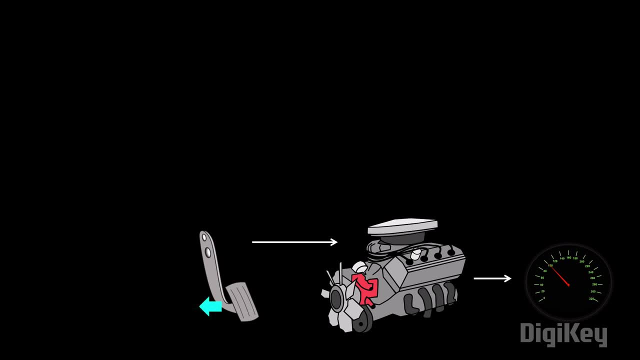 foot Press a little and some air and fuel go into the engine and your car starts to accelerate slowly and speed. Mash the pedal to the floor and you'll start dumping a lot of air and fuel into the engine. You'll accelerate quickly and at some point you will reach the maximum speed for your 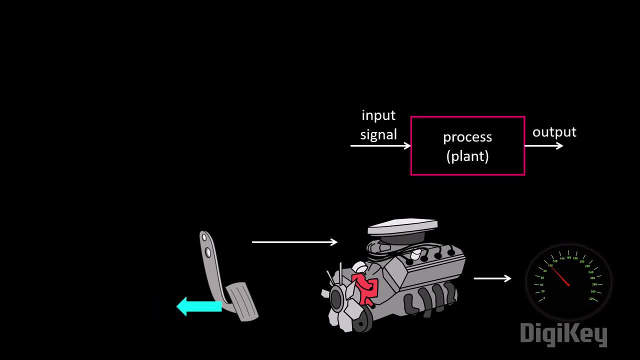 car. Our car is an example of a process or plant. We can give it an input signal, the accelerator position in this case. The car will respond with motion and we can read the speed of the car on our speedometer. That's the output. Let's say we want to maintain some constant speed, As it turns out. 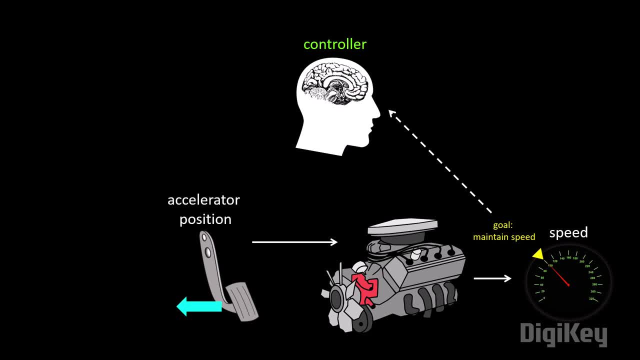 we can often read the speedometer and adjust the gas pedal as necessary to maintain that speed. Keep in mind that on flat roads you can just hold the pedal in one spot to maintain speed, but you will need to adjust the accelerator position when going up and down hills and around. 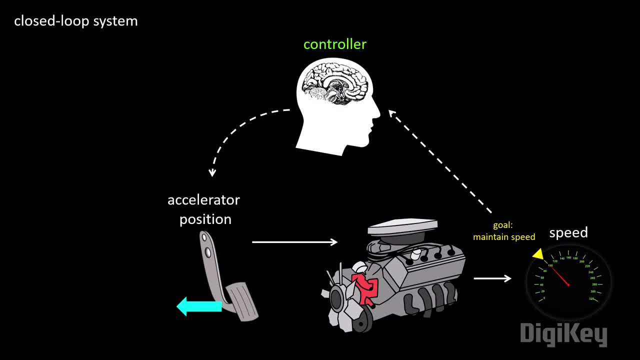 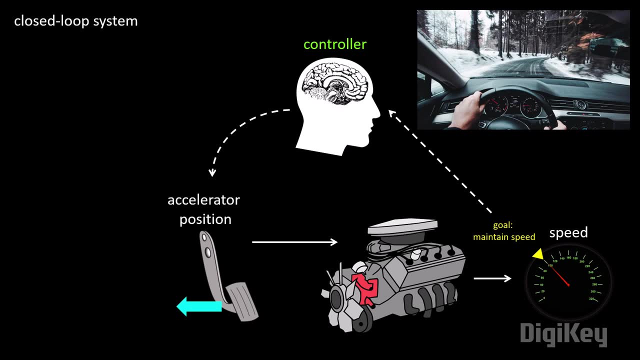 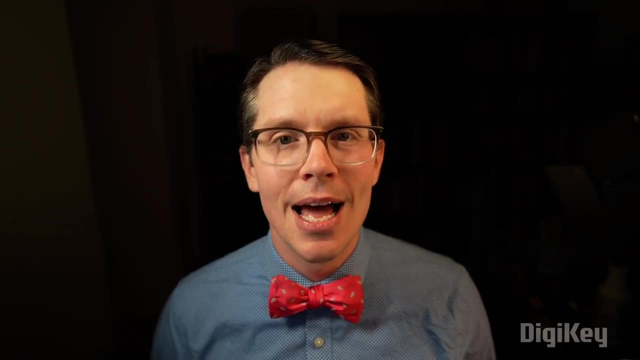 turns. This is a closed loop system. We read the speedometer, or judge speed, by looking out the windshield and adjusting the input signal- the accelerometer in this case- as needed. However, let's say that you, the engineer, have been passed with designing a controller that will automatically adjust the accelerator as needed. 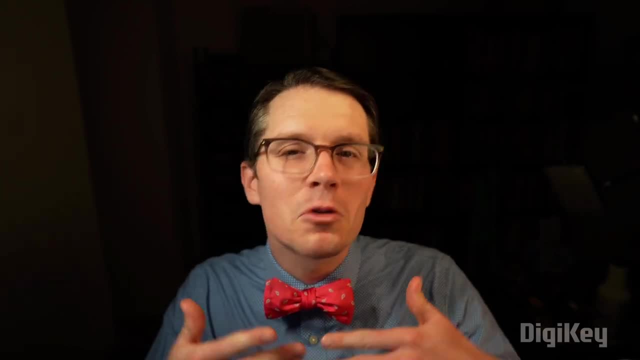 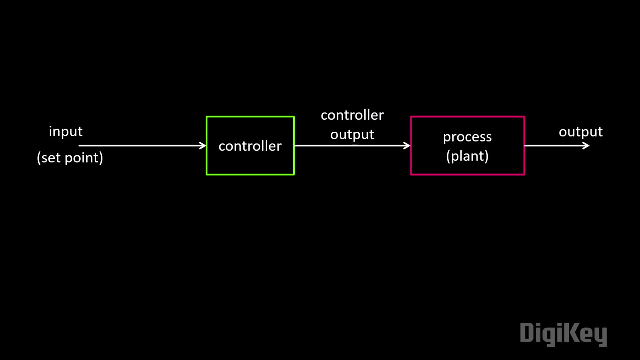 to maintain a consistent speed. We'll call this cruise control. That has a nice ring to it. Here's our initial pass at a control system. Our controller takes some input or a set point. In our example, this is like setting a particular value on our cruise control. 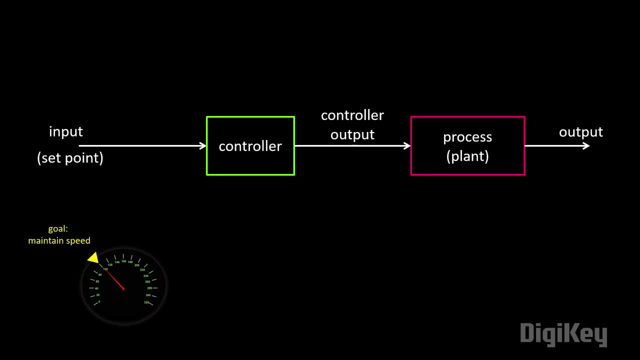 say 100 kilometers per hour. The controller then figures out what value to send to the plant. Remember that the plant is the same value as the accelerator. so it's the same value as the accelerator. The plant in our example is the engine. So let's create a simple mapping from desired speed. 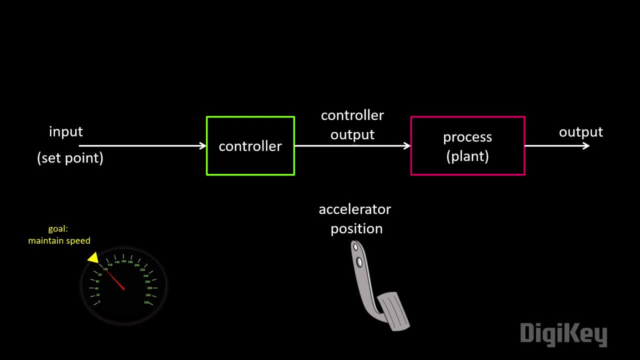 to accelerator position, as we know that the car will reach a maximum speed based on that position. The pedal position will in turn affect the engine, which will accelerate the car up to some speed. Seems simple enough. This is known as an open loop system. There is no sensor or feedback loop. 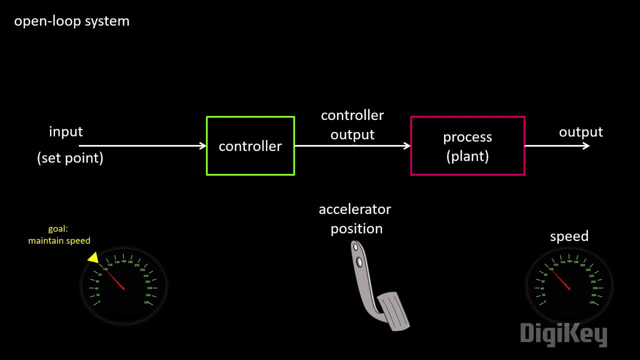 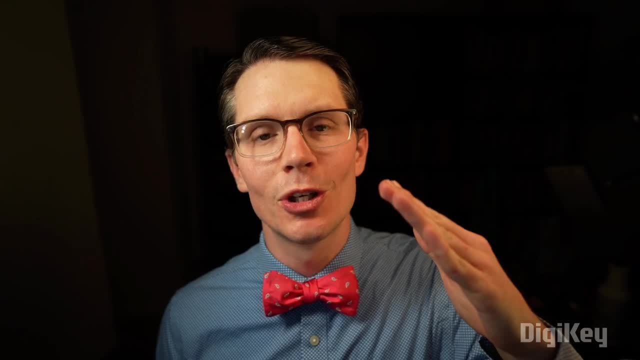 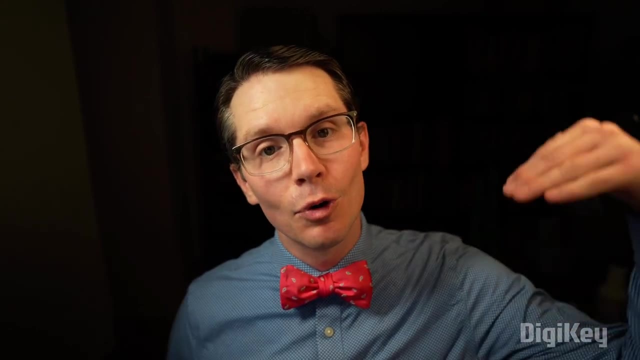 While this might work in some cases, I'm sure you can already see some issues with this control for our cruise control device. If we're going up a hill, the car is going to slow down thanks to the effects of gravity, even though the accelerator is in the same position. Similarly, if we're going 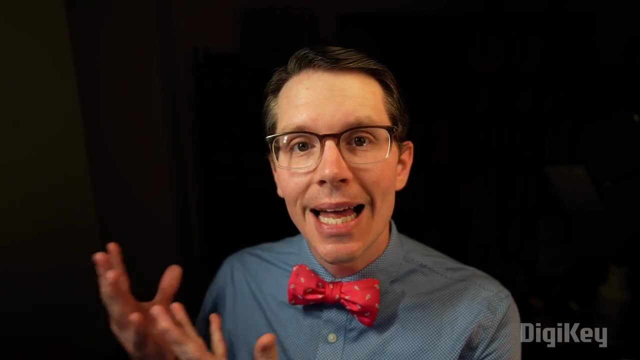 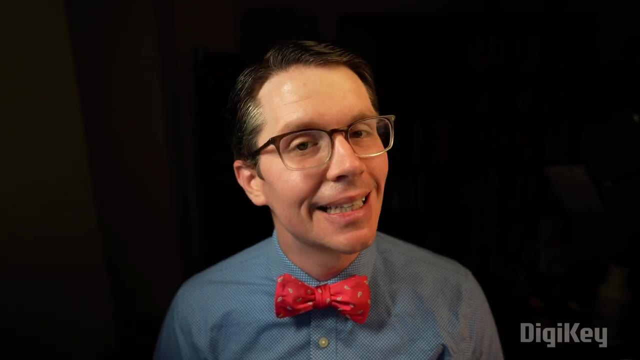 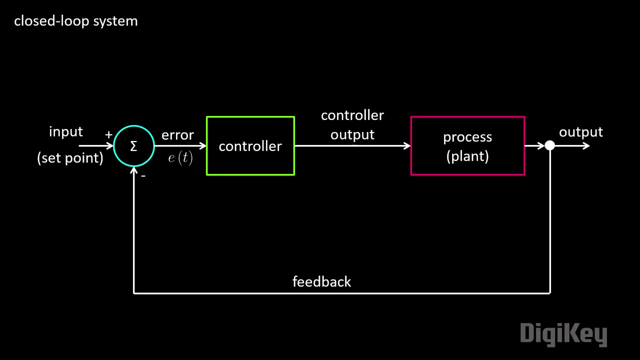 down a hill, the car is going to speed up, So we need to let off the gas pedal in order to maintain that same speed. This is something that our open loop system cannot accommodate, So we turn to a closed loop system. Here the output is measured by some sort of 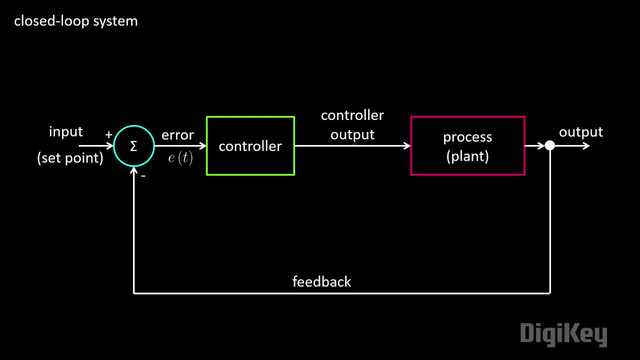 sensor and that feedback is sent to our controller. In most cases we will compare the input setpoint to that feedback to generate an error signal which goes to the controller. We'll label that error signal as E, as it's something that can vary over time. 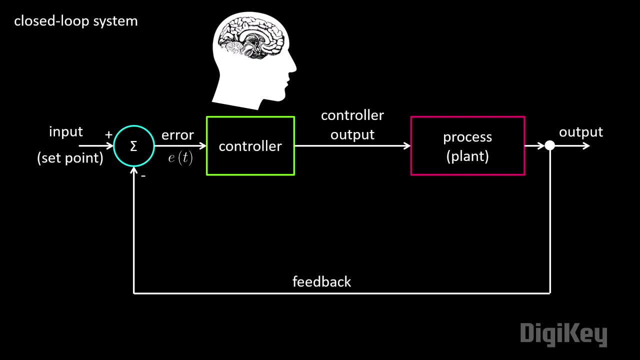 In our manual example, our brains acted as the controller. We could adjust the gas pedal with our foot as needed to maintain our speed regardless of road variations. But we want to automate this process, to take the input setpoint to the controller So we can adjust. 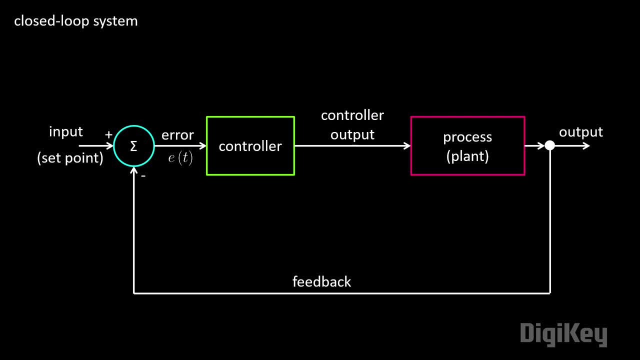 that pressure off the driver. So we need to design a controller that accepts the error signal and outputs some other signal to drive the process. First let's try simply multiplying our error value by some constant to get the output signal. This is known as a proportional controller, as the output signal is proportional to the error term. 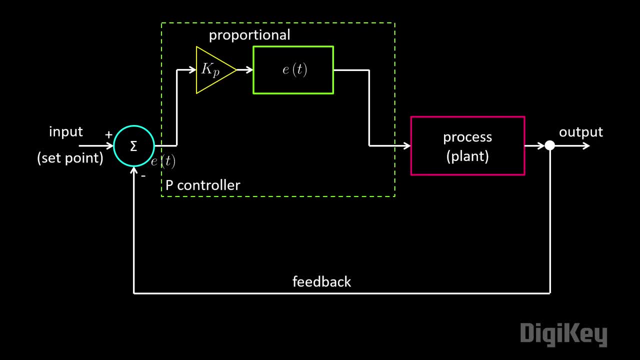 We'll start with a very simple example before coming back to our cruise control system. Instead of speed, let's say that we want to move our car 10 kilometers. Our setpoint is 10 kilometers. Our error is the difference between this setpoint and the actual. 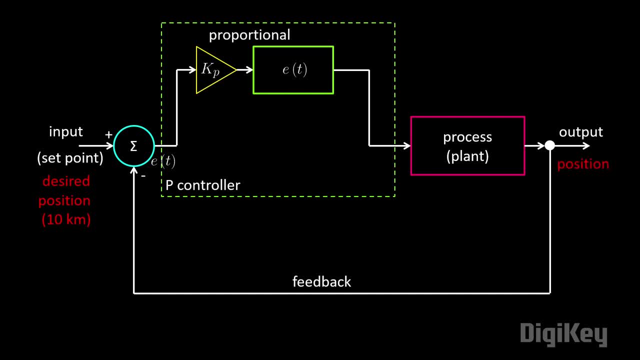 position of the car. Therefore, our error is a measurement of the distance to the goal. We want the output to be the speed of our car in kilometers per hour. The plant is still our car or engine. We give it a speed and it performs the movement for us. Here's a diagram of our car. 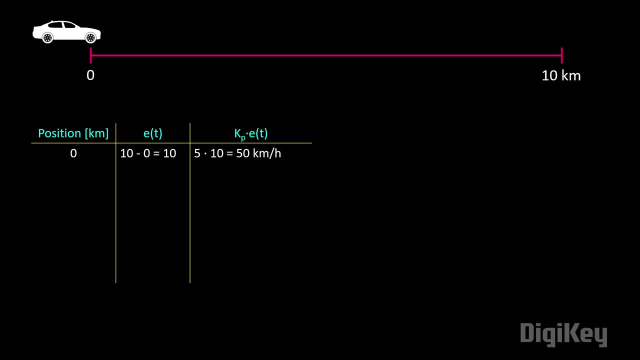 moving toward its goal At 0 kilometers. the error is 10 minus 0, so 10 kilometers. Let's set our constant kp to some arbitrary value like 5.. So we multiply 5 by that error to get our controller. 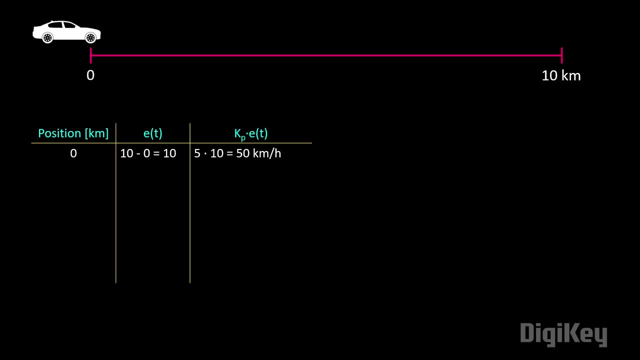 output, which is 50 kilometers per hour, Our car starts moving very quickly at first. Don't worry about acceleration and deceleration. for this very simple example, At 3 kilometers the error is 7 kilometers, so our speed slows to 5 times 7, or 35 kilometers per hour. 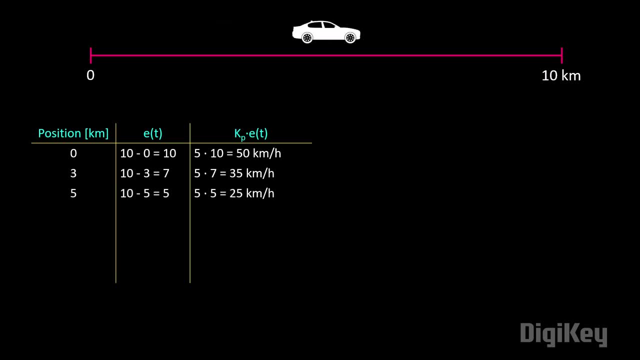 We continue with this pattern. At 5 kilometers, the speed is 25 kilometers per hour, as the error is 5 kilometers. At 7 kilometers, the error is 3, so the speed slows even more to 15 kilometers per hour. Similarly, at 8 kilometers, the speed drops to. 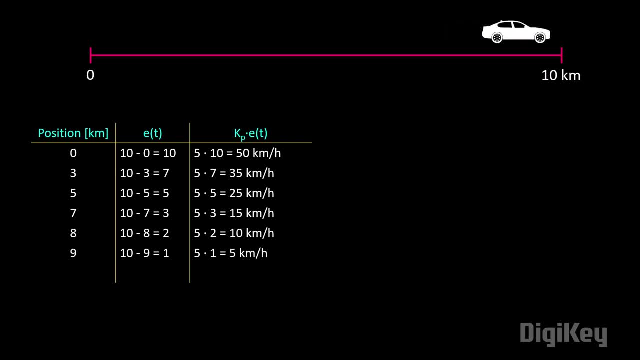 10 kilometers per hour And at 9 kilometers the speed slows all the way down to 5 kilometers per hour. Finally, at our goal, the speed should be zero kilometers per hour, as our error is zero kilometers. If we graph our error and speed, we should see something like this: 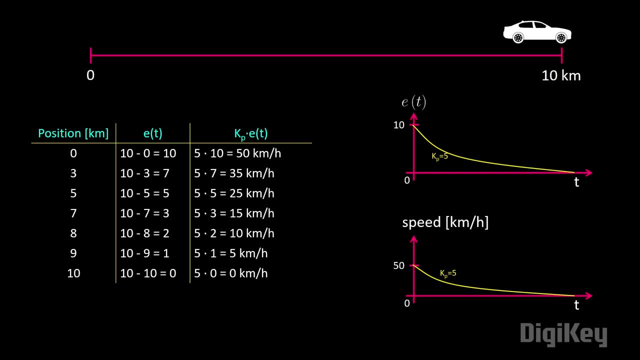 The error starts at all kilometers per hour. When we egg it all in, the error lasts 5 kilometers per at 10 kilometers, and the speed is proportionally high at 50 kilometers per hour. As we get closer to our goal, the speed also starts to drop. 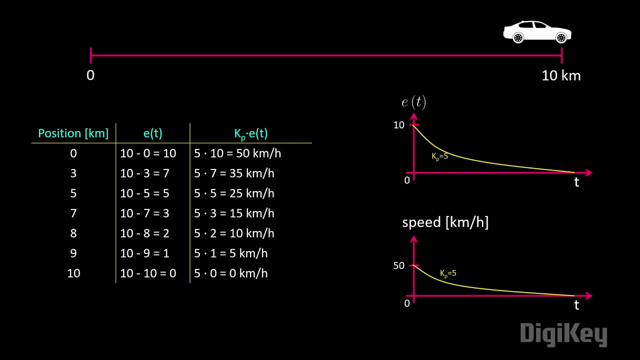 As a result, we approach our goal more slowly until we're barely moving at all. Assuming an ideal system, we should reach our goal at a snail's pace without overshooting. Note that we can adjust our constant value. For example, if we set it to 2, the speed will be slower, but still proportional to. 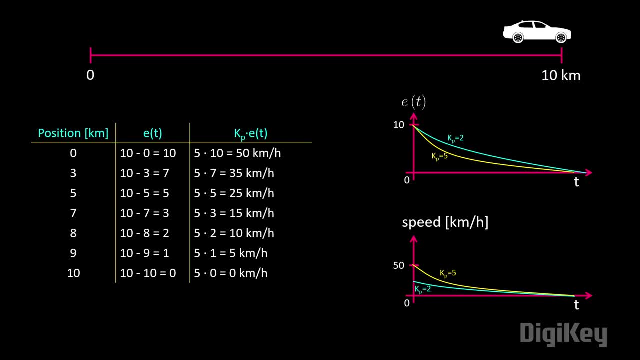 the distance error, It will take longer to reach our goal. If we increased the constant to say 10, we'll reach our goal much faster, But we start risking overshoot in non-ideal systems and possibly breaking some speeding laws. 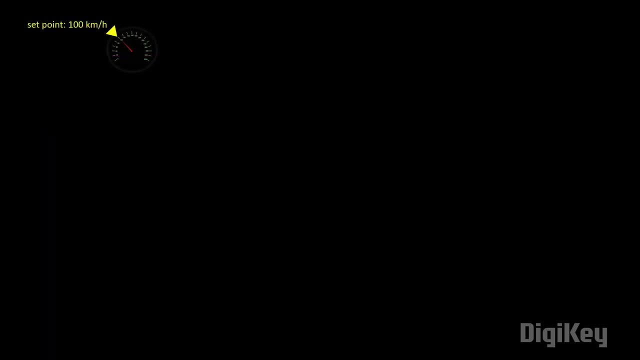 Now let's turn our attention back to the cruise control system that we're designing, as it's a little more complex than this distance problem. Remember, we want our car speed to match our setpoint at 100 kilometers per hour, and we 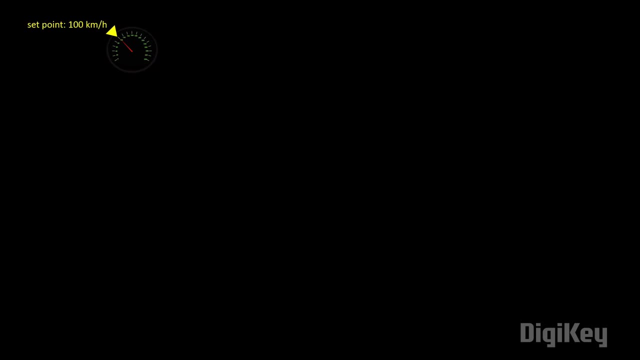 need to design a controller that can take in this information and adjust the accelerator position. We'll say our accelerator position can go from 0 to 10 centimeters. Zero is when we're not touching the pedal and 10 centimeters is pushing it in as far. 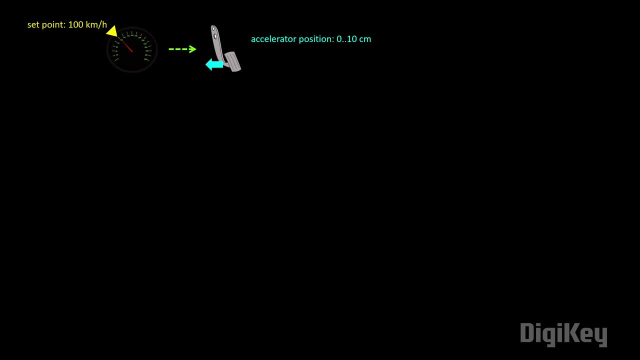 as it will go. For the sake of argument, we'll say that we can cruise at 100 kilometers per hour on a flat road when the accelerator is pressed in at 5 centimeters. Now let's choose an initial proportional constant, say 0.1.. 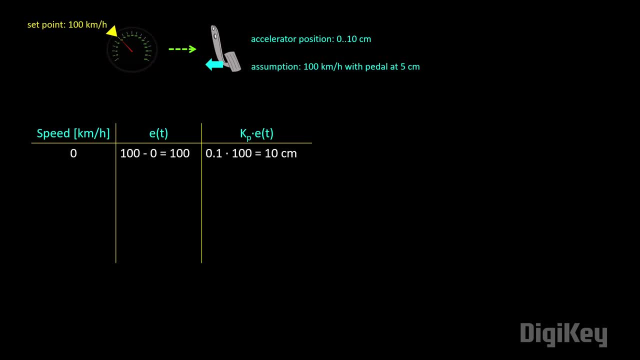 0.1.. 0.1. Over 5-ch곰ème. The error is means 100 kilometers per hour and the output of our controller is 0.1 times 100.. That's pressing the accelerator all the way in, so we will accelerate quite quickly. 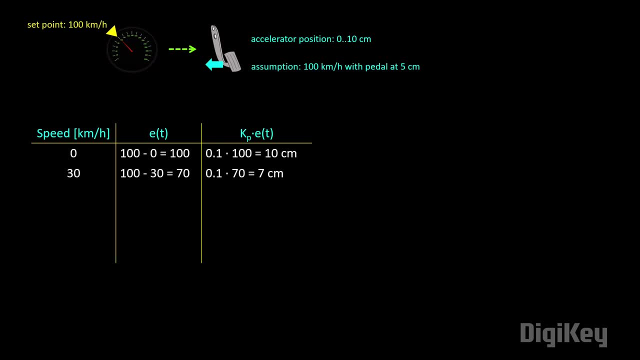 at first, then at 30 kilometers per hour, our error is 70. Time is our constant of 0.1, and that means we begin to let off the gas pedal by a few centimeters—at 50 retired kmh, we've moved the gas pedal to 5.10kms. 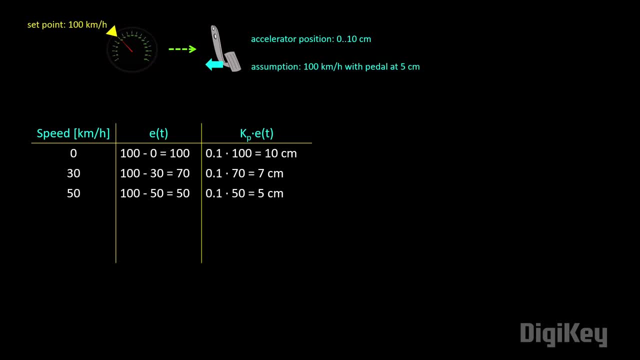 That's our assumed setting, so 0.1.. cruising pedal position. Do you see the problem? We're not at our desired speed. At 50 kilometers per hour and a pedal position of 5 centimeters, we'll continue to accelerate some. However, once we reach 60 kilometers per hour, our 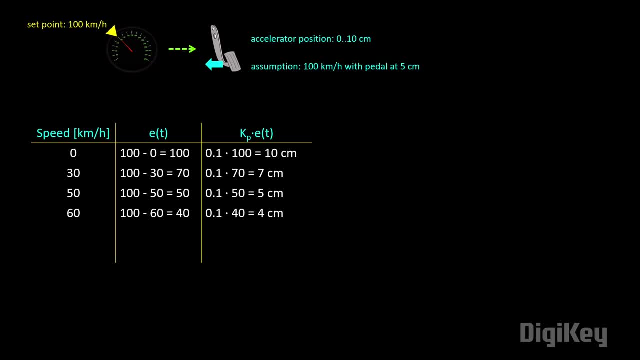 pedal position will be at 4 centimeters. For the sake of this example, we'll say that we can cruise at 60 kilometers per hour with the pedal position at 4 centimeters, but we'll never quite get to our desired speed If our error is 0,. 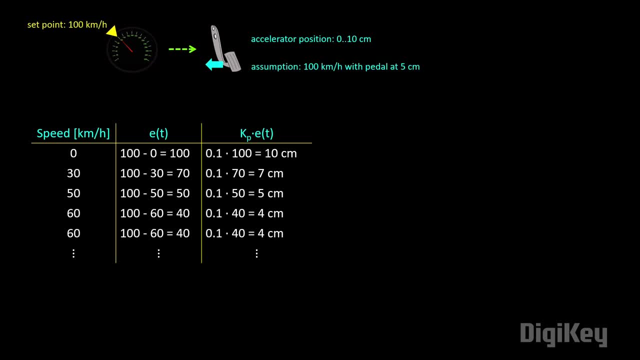 that means our proportional controller will set the accelerator position to 0, which essentially means no power from our engine. Let's graph our error and speed. As you can see, we go from 0 up to 60 kilometers per hour, but we never. 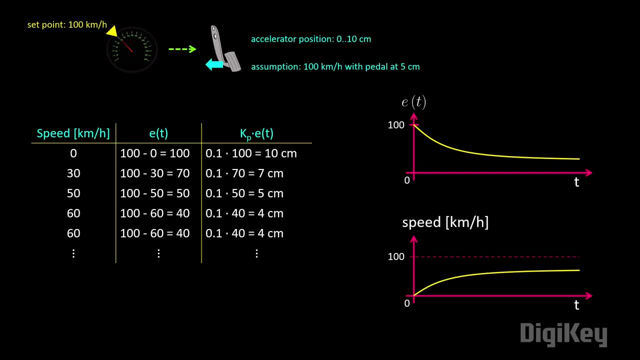 quite reach our setpoint. The difference between our setpoint and actual achieved cruising speed is known as the steady state error. Many systems, like a cruise control, suffer from this steady state error. No matter how we adjust kp, we'll never quite get to the setpoint We could. 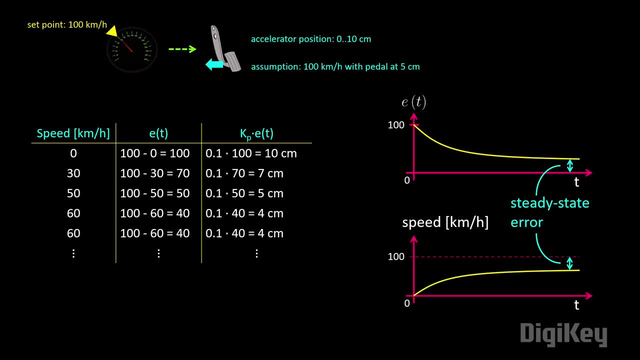 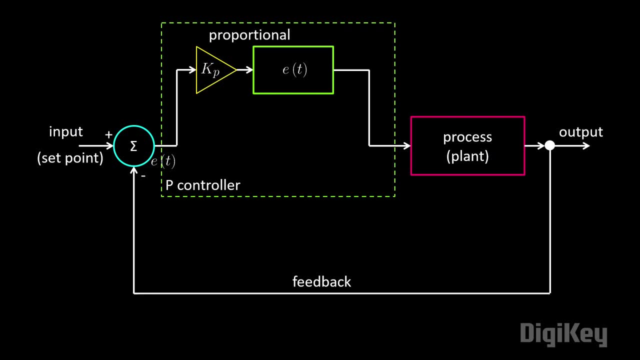 include a constant offset, but there's a better, more robust way to handle such errors. Let's go back to our system diagram for a moment. A common way to find steady state error is to look at how much error has accumulated over time. 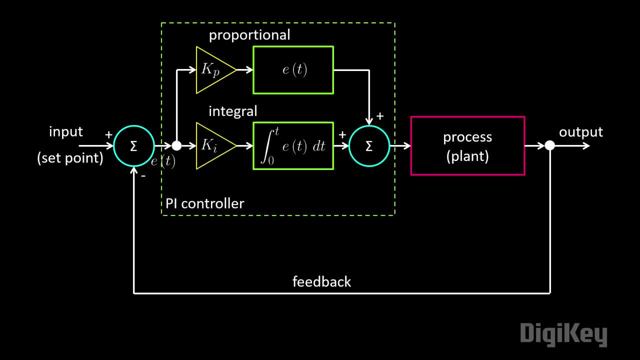 We then multiply that amount by some new constant, ki, before adding it to the value of our proportional controller. In the math world, we would take the area under our error curve, which would be an integral. This is how we get to a PI. 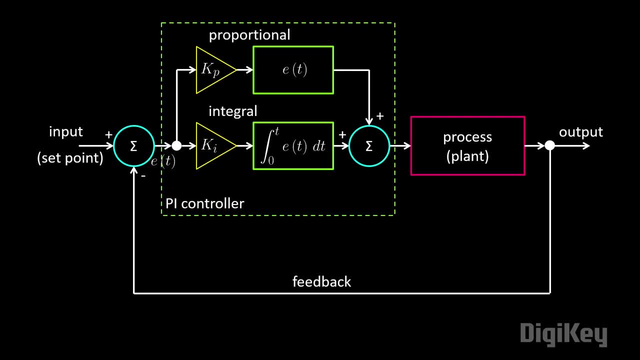 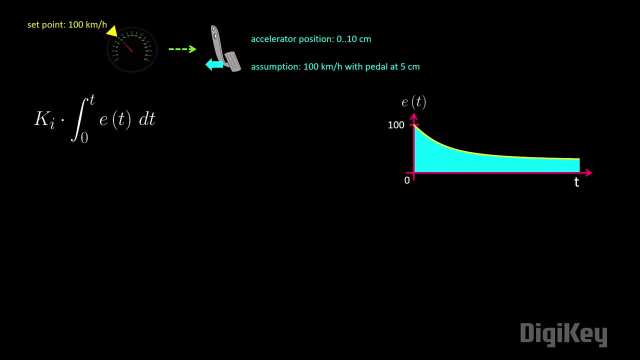 controller. Proportional and integral values are summed together to produce a single output. However, integrating this unknown error function is often impossible for most real-world systems. So we can take an approximation of that integral. We simply sum each error term over time and then multiply that. 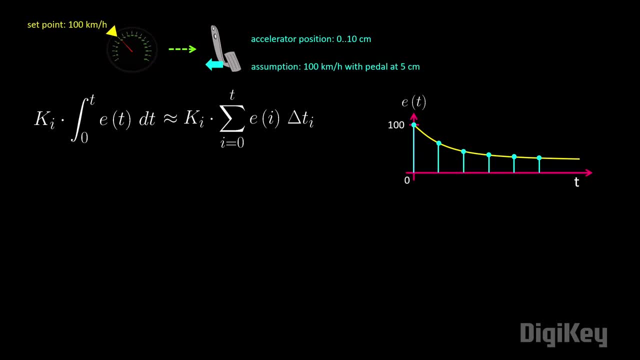 accumulated value by our integral. Now let's see what happens if we include this integral term with our proportional term. Let's say that this integral term is constant and we want to multiply it by a delta t interval time To make our calculations easier. we can assume that this is 1.. 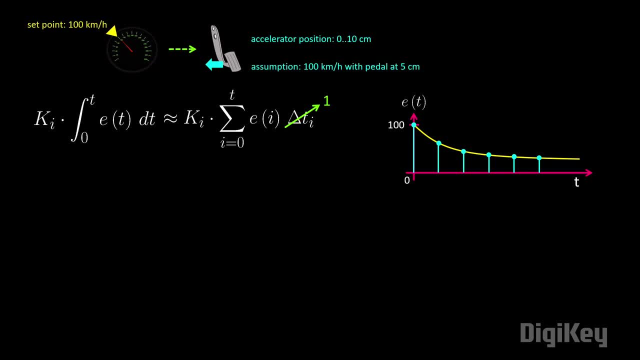 For example, maybe we take an error reading every one second, Or if we know that this interval time is constant, we can just say it's part of our ki value. Either way, we won't need to worry about this term in this example. 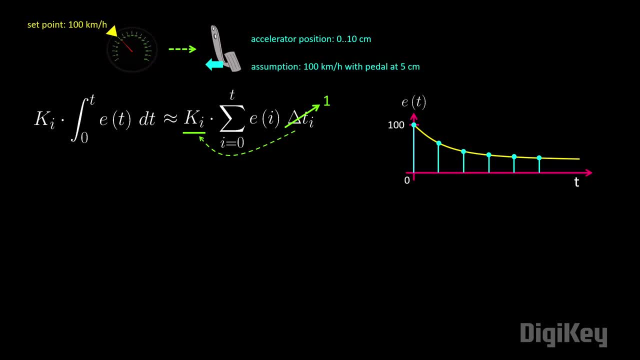 Now let's see what happens if we include this integral term with our proportional term. from the previous example, We start at 0 km per hour, so our error is 100.. From before, we know that our proportional controller wants to set the. 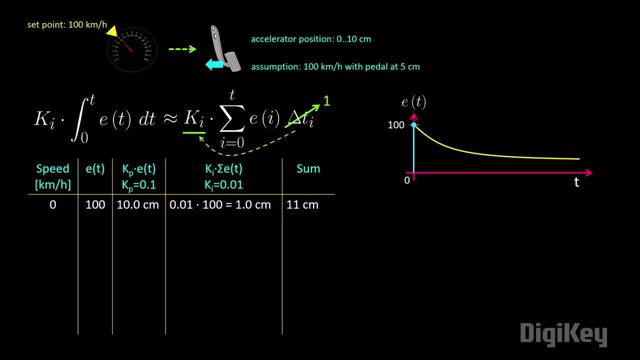 accelerator to 10 cm, assuming we have kp set to 0.1.. We'll set the ki term to 0.01.. As this is the start of the accumulation, the approximate integral is just 100.. 100 times our ki of 0.01. 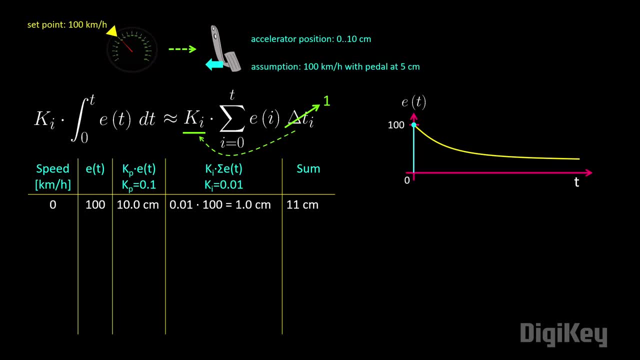 is 1 cm. We then add the two controller outputs together to get a sum of 11 cm. Our accelerator doesn't go to 11, so for now we'll just say we max out the accelerator at 10 cm, We start accelerating up to 30 km per hour. 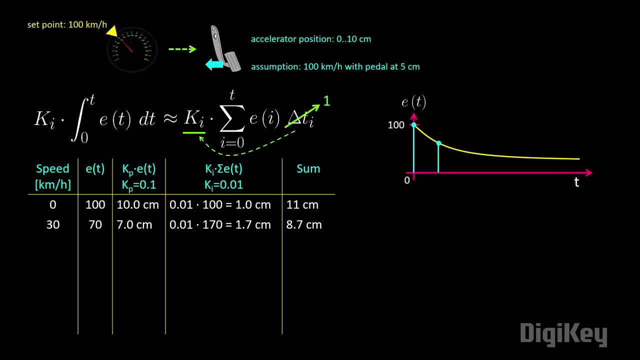 so our error term is now 70. Our proportional controller sets the pedal to 7 cm. In the integral controller we accumulate 70 on top of 100 to get 170, and multiply that by our constant to get an output of 1.7 cm, Our new PI controller. 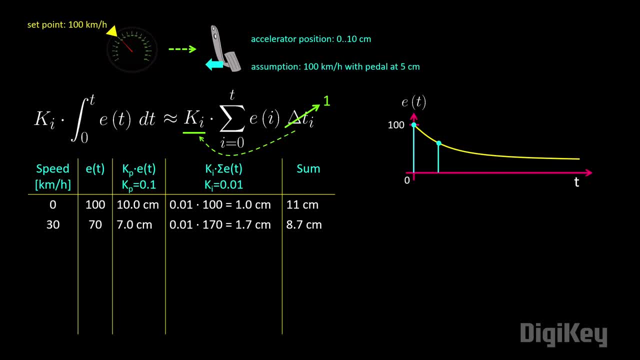 output is 8.7 cm, so we keep the accelerator pressed farther than we did with just the P controller. We continue this trend to get a PI controller output of 7.2 cm when going 50 km per hour. Notice that the P controller is starting to contribute less, but the I controller. 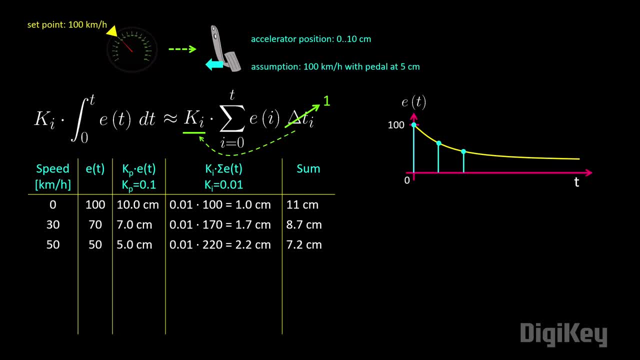 is contributing more as the area under the error curve grows. At 70 km per hour, the output is 5.5 cm. We've already passed our original limit of 60 km per hour when we used just the P controller, Even at 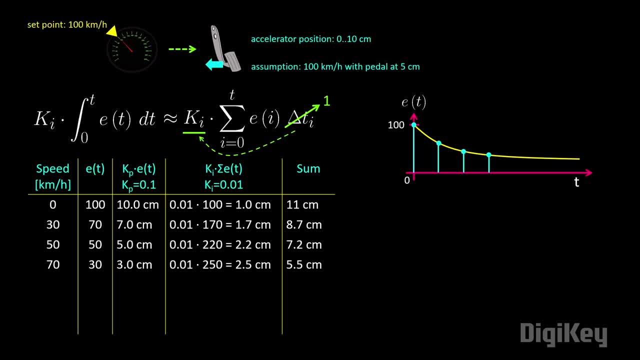 70 km per hour, our controller is saying to continue accelerating. However, when we reach 80 km per hour, the total output has dipped below 5 cm, which we know is a problem. There's still an error, But wait, let's see what happens. 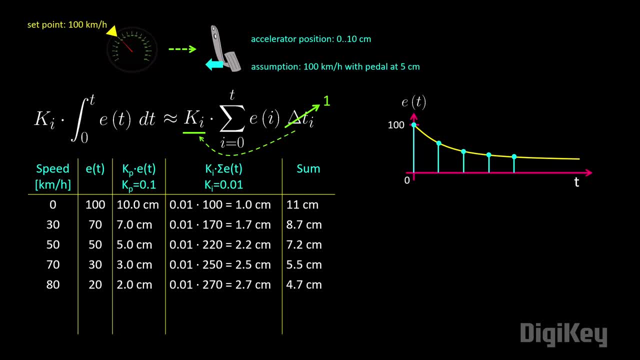 next, Assuming we continue at 80 km per hour, the P controller will output the same amount. However, the integral controller continues to accumulate. It says to increase the value of the output to account for that error. So we press the accelerator a little more to start closing that error. It might look like the output. 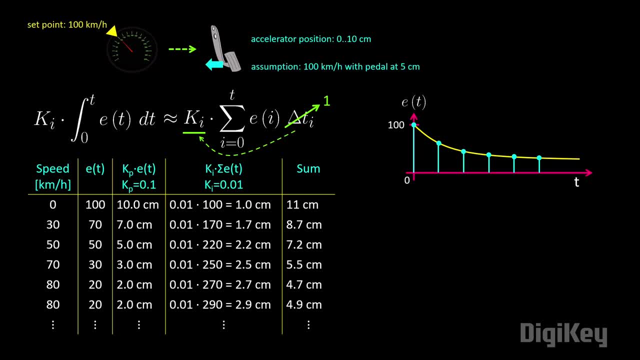 will fluctuate as it approaches that steady state value. but this example is just intended to show how the integral controller will account for that error. In reality, our example will look something like this: The proportional and integral terms will reach a steady state when the error is 0, which. 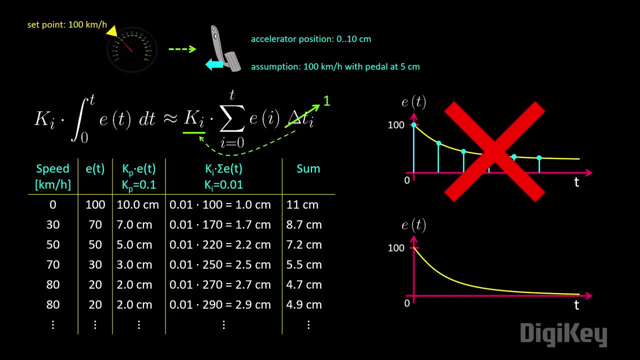 means we perfectly hit our mark. In fact, in many cases, a PI controller is all we need. It's enough to move a process toward its goal, while accounting for steady state error. However, you'll often run into other issues that can't be solved by proportional and integral terms alone. 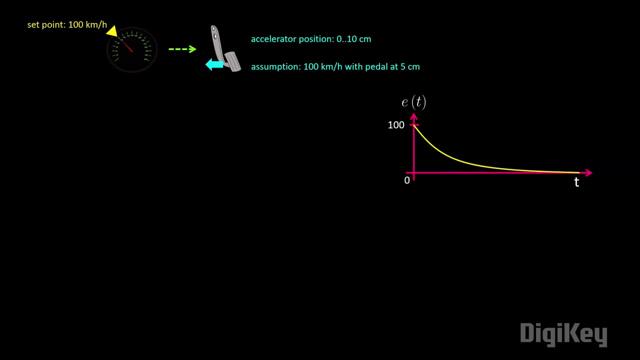 A well-tuned PI controller looks something like this. However, the rate of change might be too slow for you. This is known as an overdamped response. You may want your process to approach the goal quickly, So you start playing with the KP and KI terms. 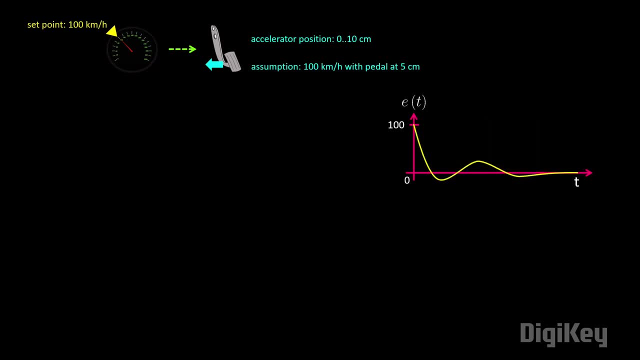 and you end up with something like this: While the system approaches the setpoint quickly, it also overshoots. The integral term will account for the negative error and eventually bring the output in line with the setpoint. However, the system might oscillate for a while before it does that. 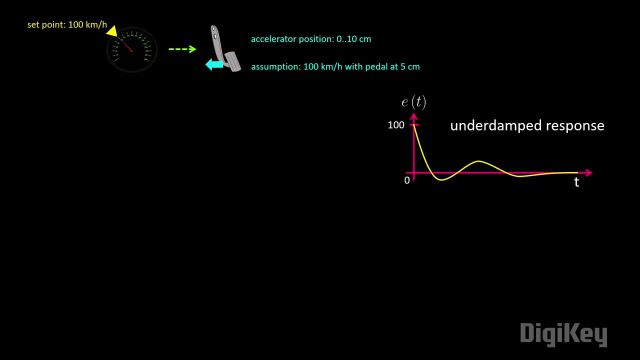 This is known as an underdamped process. In many cases, no matter how much you fiddle with the KP and KI terms, you can't seem to find a good balance between an overdamped and an underdamped response. What you're after? 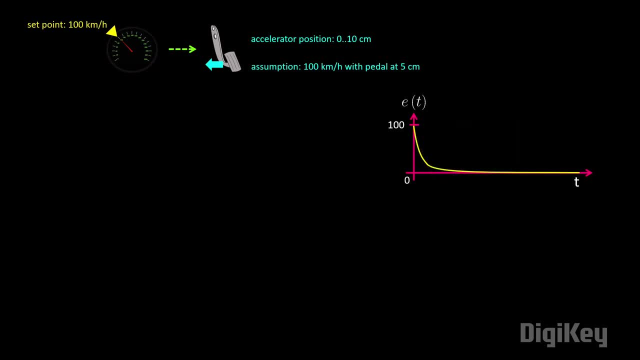 is a response curve that looks like this: The process quickly approaches the setpoint and settles there with no overshoot. This is known as a critically damped response. To make this happen, we need to add one more component to our controller. This is the derivative term. 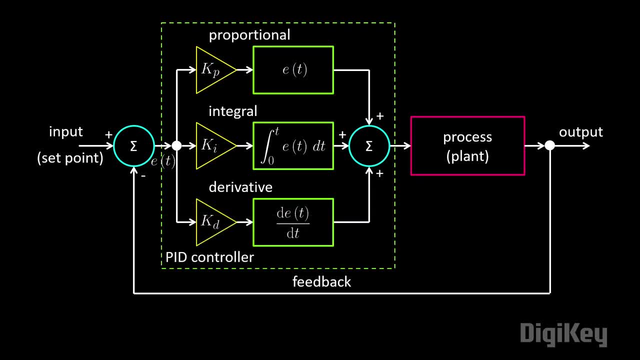 We multiply the rate of change in the error by some constant kd. We sum the proportional, integral and derivative terms together to get the output. This is known as a PID controller. Let's see how this works with an example: The derivative of the error. 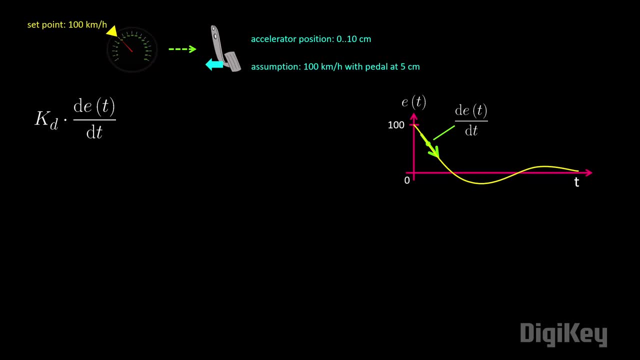 is the slope at that particular point. That means if the error is decreasing quickly, meaning we are accelerating fast toward our target speed, then the derivative term will be a negative number with a large magnitude, Like with the integral term. this is often difficult or impossible. 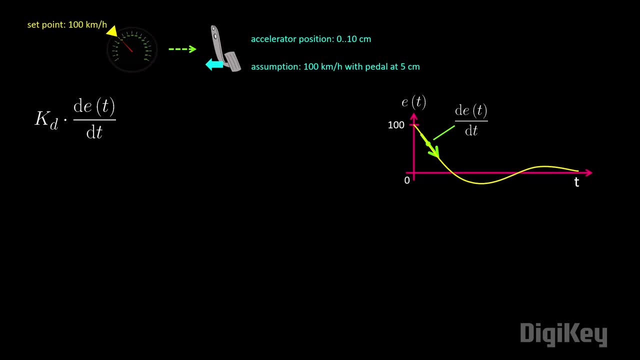 to analytically solve unless you have a mathematical model of your process. So we turn to numerical estimations again to help us out. We can approximate the derivative by simply subtracting the current error value from the previous error value and dividing that by our. 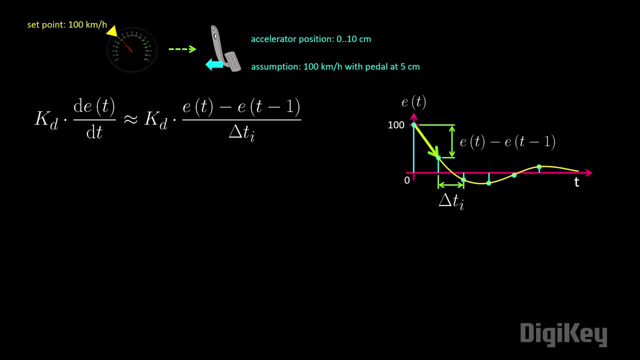 sampling interval time. That should give us the slope of the line between the current and previous values, which is good enough for what we need in most cases. And, just like we did with the integral term, we can assume the sampling interval delta t is 1, or we can assume it's part of our constant. 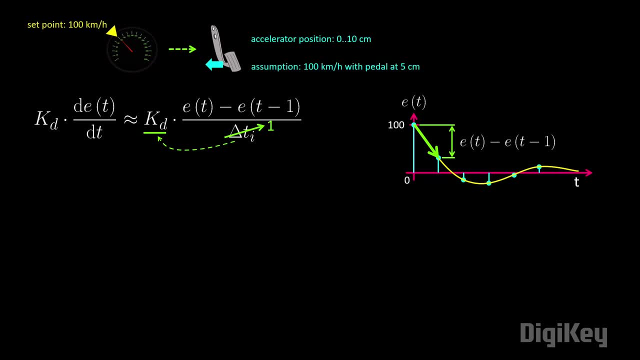 for now, The difference between the current and previous error values will work in this instance. The idea is that we want a term that can tell if we are approaching the goal too fast and dampen the response just enough so that we don't overshoot. So let's work on. 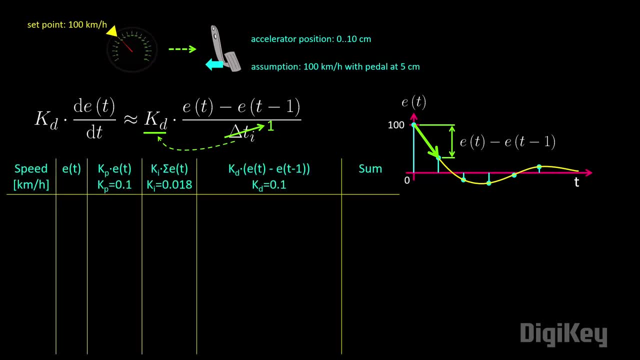 another simple example. Here we've added the proportional, integral and derivative terms. I've adjusted the ki coefficient to be a little higher. That way our speed increases much more quickly toward our goal, at least in theory. It's not a perfect example, but it should illustrate how the p, i and d 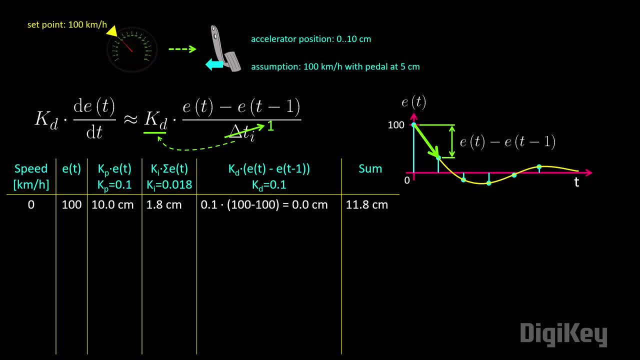 terms work together. At first we accelerate very quickly from a stop. Note here that the derivative term is 0,. as we do not have a slope yet, Once again, we make the assumption that we can only push the pedal to 10 centimeters. 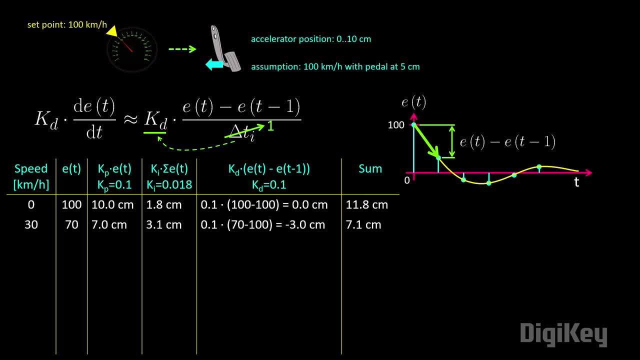 At 30 kilometers per hour, the integral term starts to increase quickly. However, because we are accelerating so fast, the difference between this and the last error terms dampen the current pedal position to 7.1.. We repeat this procedure and we see. 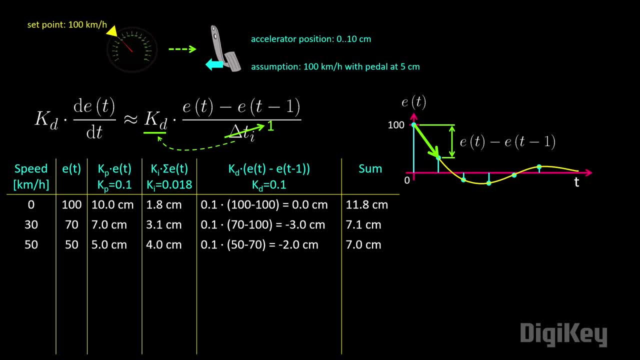 that we've dampened the pedal position again to 7 centimeters. At 70 kilometers per hour our derivative controller output is again minus 2 centimeters, which makes the total 5.5 centimeters. We still have the pedal pressed more than what we want to cruise at. 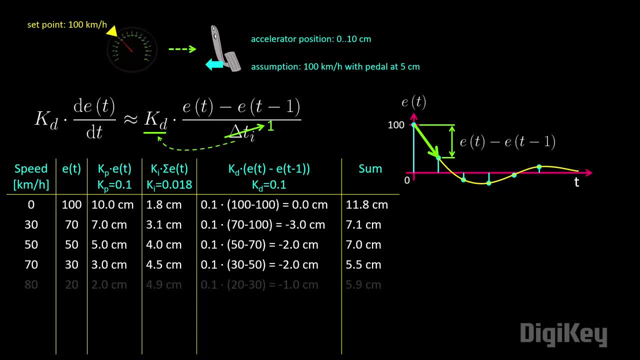 but it means we're accelerating As we start to approach our goal. you can see how the proportional term approaches 0, and the integral term takes over. The derivative term is no longer needed to dampen, so that also approaches 0. In the ideal case, we land right. 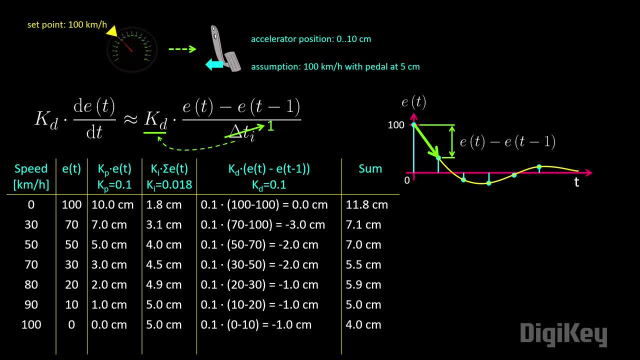 at 100 kilometers per hour with the pedal at 5 centimeters. We probably overshot a little, as the pedal was pulled back to 4 centimeters for that second-to-last sample. That's probably just indicative of my poor example here. However, it shows that we need to tune the. 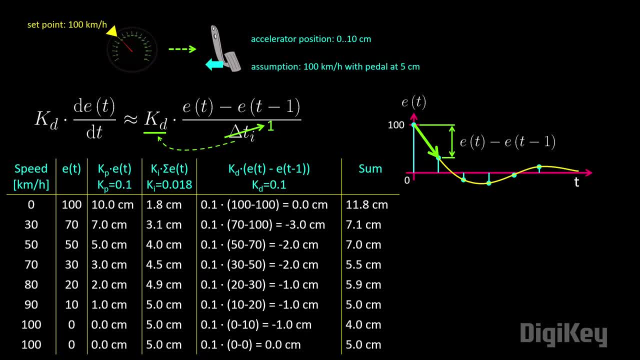 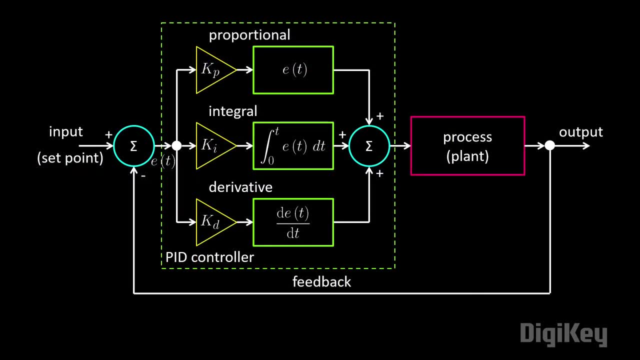 Kp, Ki and Kd terms to make a system that is critically damped, where we approach our goal quickly without overshooting. If you have a mathematical model that correctly describes the behavior of the plant, you can solve for Kp, Ki and Kd. 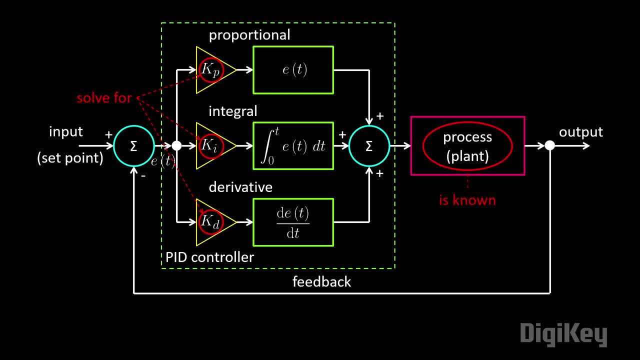 to make the system critically damped. This model is usually expressed as a transfer function, which gives the plant's output for any given input. This works well in academic settings with simple plants. In most cases it's either impossible or very difficult to know the exact. 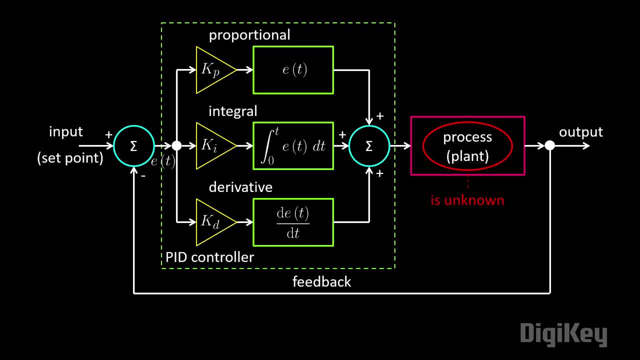 transfer function of the plant. So we turn to other tuning methods. There are a number of ways to tune a PID controller, but we'll demonstrate a simple manual method here. We measure the output as we vary each of the constants. You set Ki and Kd to 0. 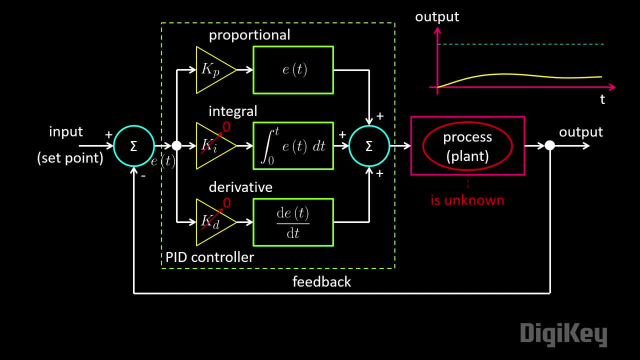 and leave Kp at some low value. You increase Kp until the output oscillates with some steady state offset. You then increase Ki until you correct the steady state offset, even if that means more oscillation. Just make sure the output does not become. 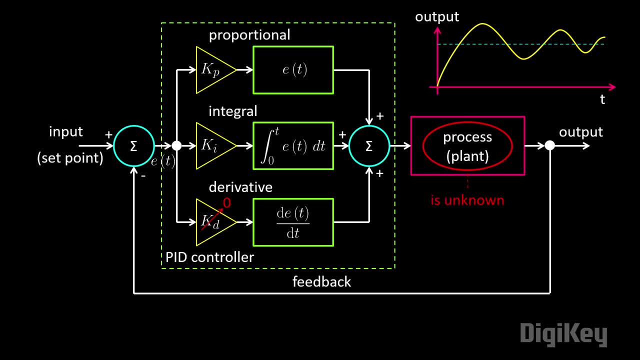 unstable and oscillates out of control. Finally, adjust Kd to remove the oscillations. At the end of the process you should have an optimally tuned system. Note: there are other tuning schemes, such as the Ziegler-Nichols method. 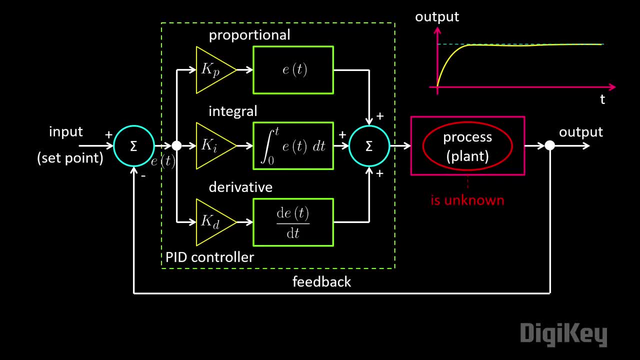 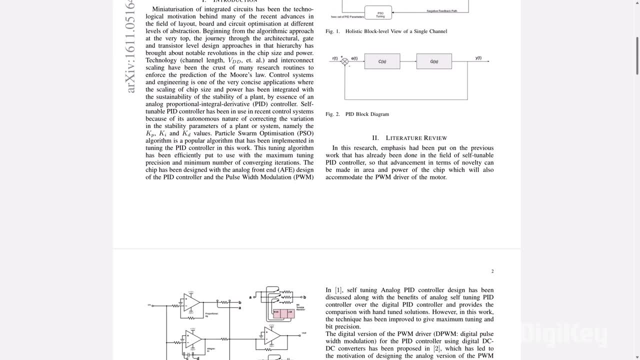 where you can use some math to help you choose Ki and Kd to reduce the amount of trial and error that's needed. Early PID controllers were pneumatic and then eventually electrical. Here is an example of a classical electrical PID controller used in a research paper. However, most 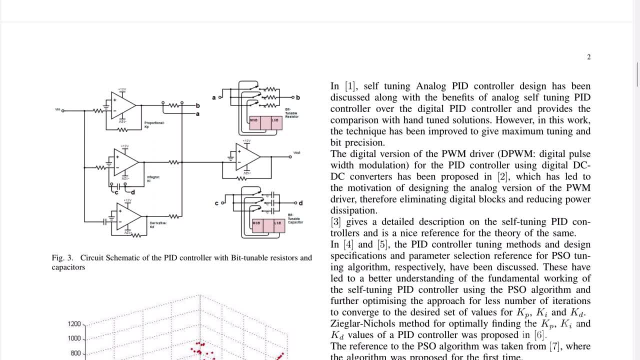 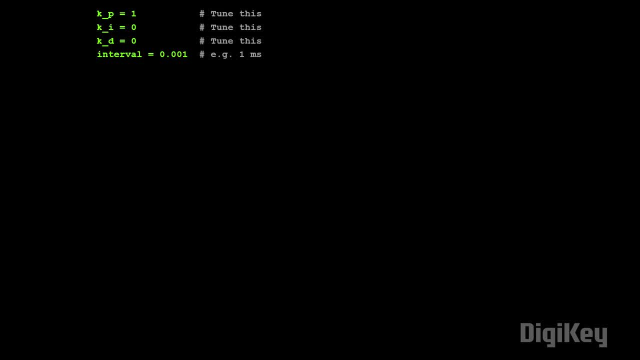 modern PID controllers rely on code and microcontrollers rather than discrete components. This is some pseudocode for how you might implement a PID controller. We set the constants to some arbitrary values to be tuned later, and we also need to know the interval time. This 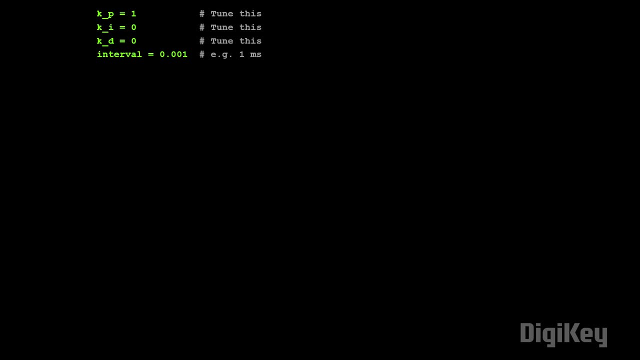 corresponds to the sample rate, how often we will sample from our sensor and perform some action on our plant. We'll go with one millisecond. We loop forever. in this case, At the beginning of the loop we read our feedback value, which is often from a sensor. We then calculate. 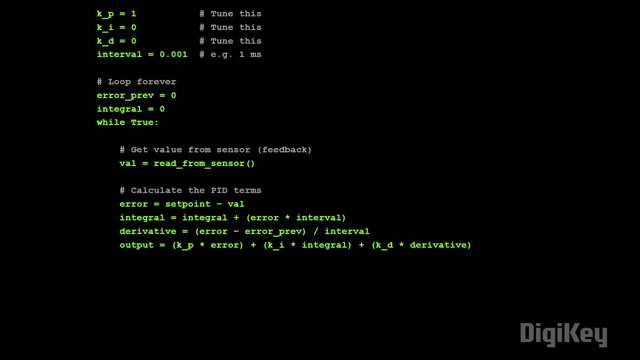 each of the PID terms. To do that, we take the difference between the set point and the measured value to get the error term. We then multiply it by the interval to accumulate in the integral term. The derivative term takes the difference between the current and previous errors and then divides that value. 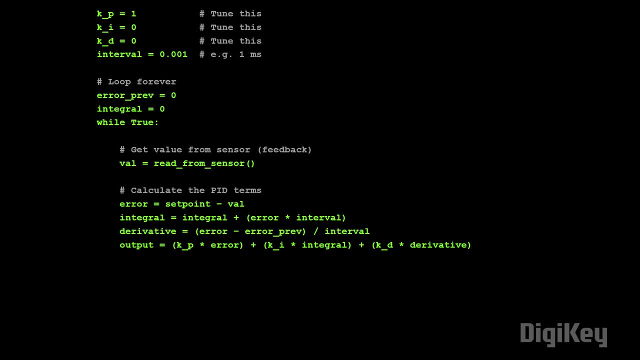 by the interval. We then multiply each of these values by their respective k constants and add them together. While not shown here, you would use that output value to drive whatever you needed. This could be say adjusting the accelerator by some amount in centimeters. 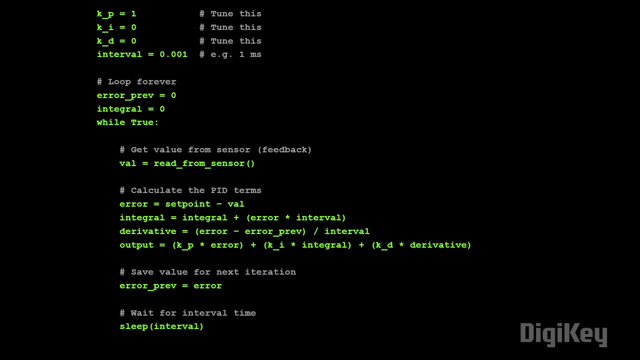 Finally, we save the error value for the next iteration and then wait for the given interval time. This is a very simple example. You could obviously do this in a separate thread with timers or using a variable interval time. You would also need to spend. 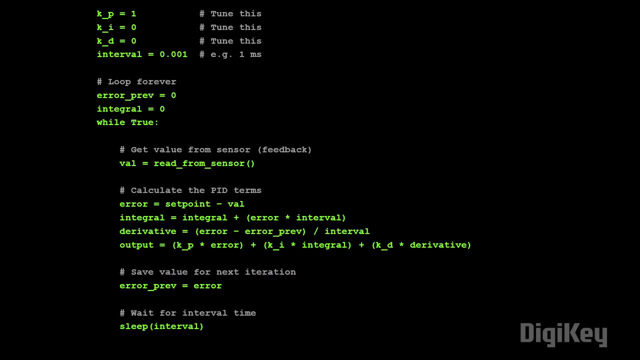 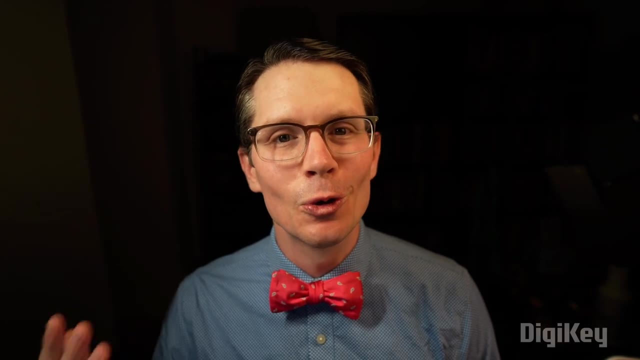 some time tuning the three k constants, but this should be enough to get you started making your own PID controllers in code. Now, where would you actually use such a controller? PID controllers are used in countless applications and, as you probably guessed, most cruise controllers are used in cruise controllers. 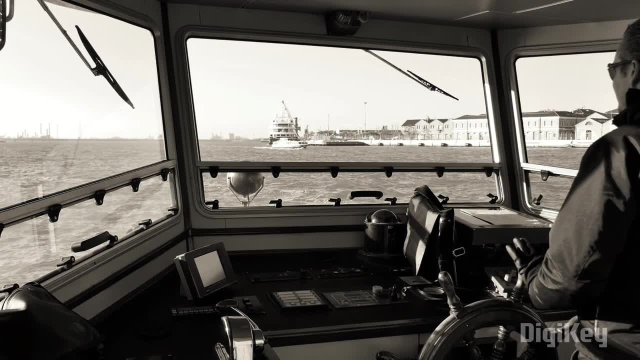 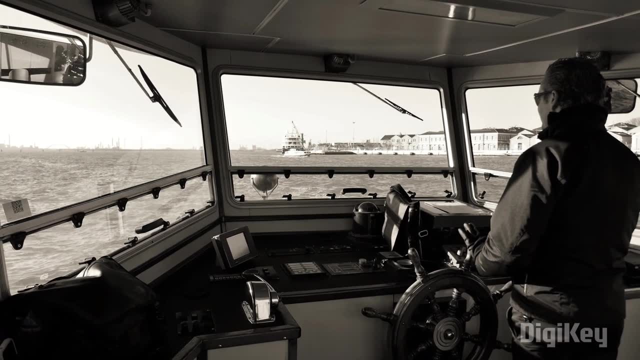 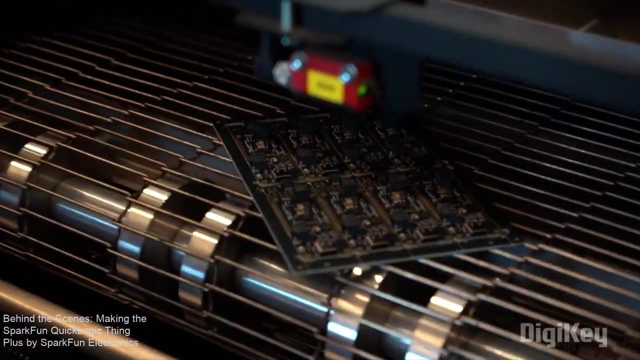 In the 1920s, Minorski was researching methods for automatic ship steering when he devised his theoretical analysis of PID controllers. They are also heavily used in manufacturing and industrial equipment. For example, many reflow ovens use PID controllers to adjust the 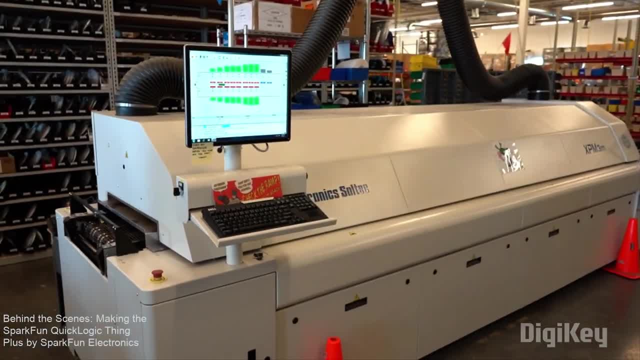 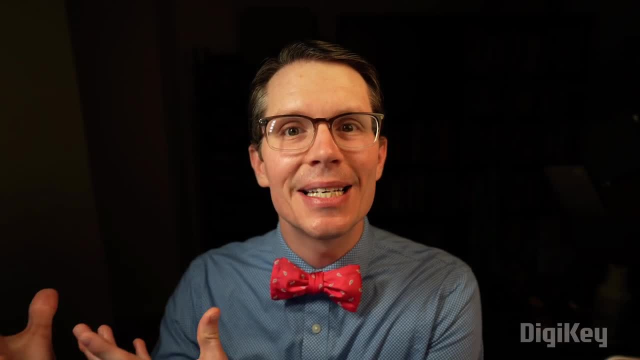 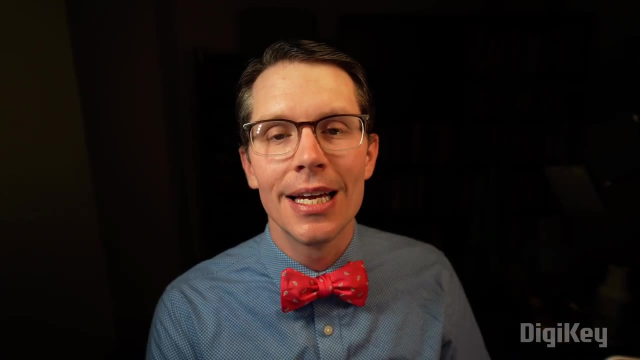 heating elements as needed to match the set points in the profile. This allows mass soldering of components without burning boards. I hope this helps you understand the theory behind the PID controller And how they can be used to regulate a system based on feedback from one or more sensors. 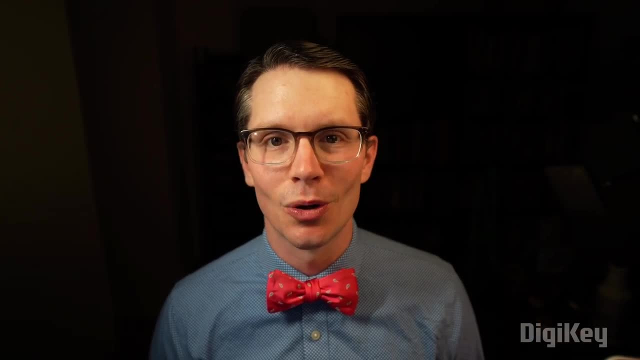 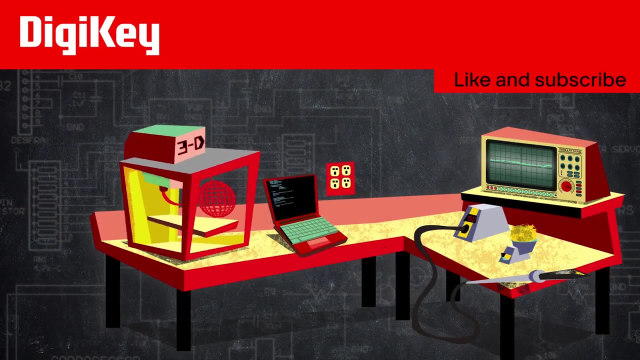 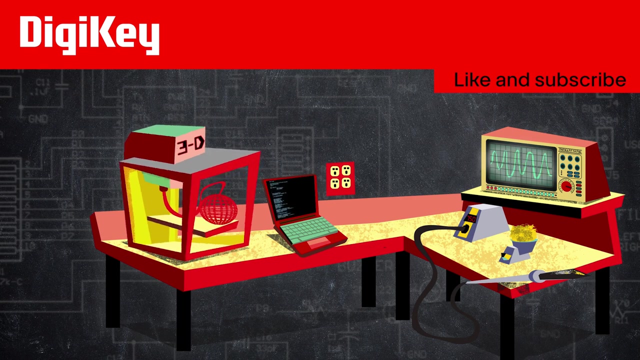 In a future episode I'll demonstrate tuning a PID controller. Stay tuned and happy hacking. Thanks for watching. 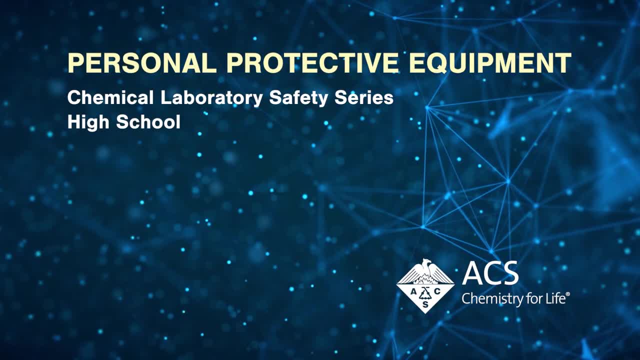 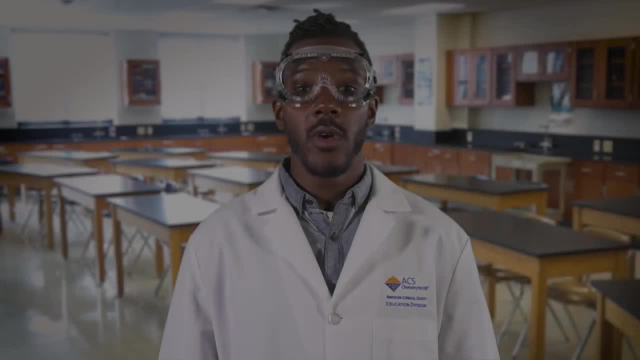 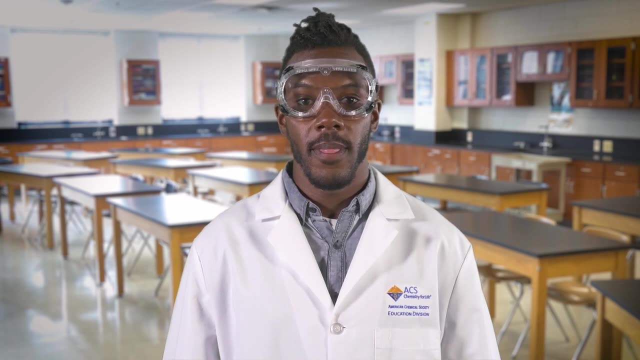 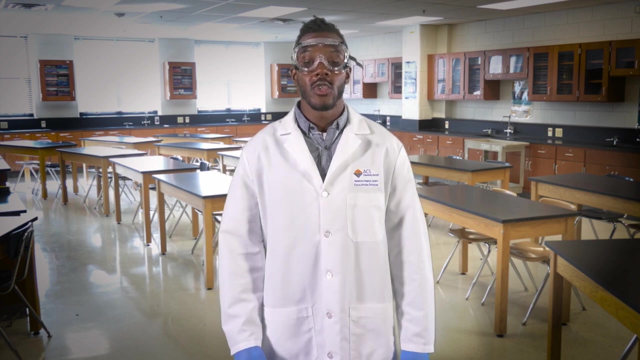 Wearing personal protective equipment- PPE for short- is one of the main ways to protect yourself from injury in the lab. PPE includes things like goggles, gloves, lab coats or aprons. These are designed to protect your eyes, hands and skin, as well as your clothing. 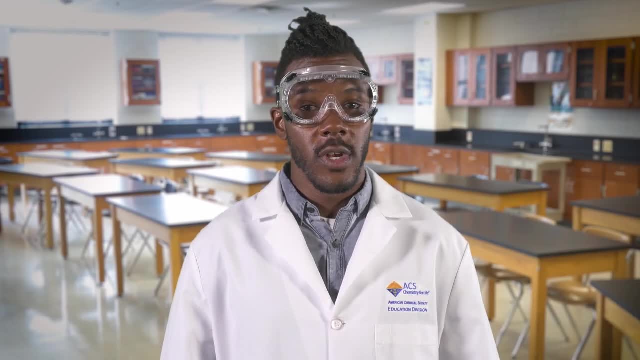 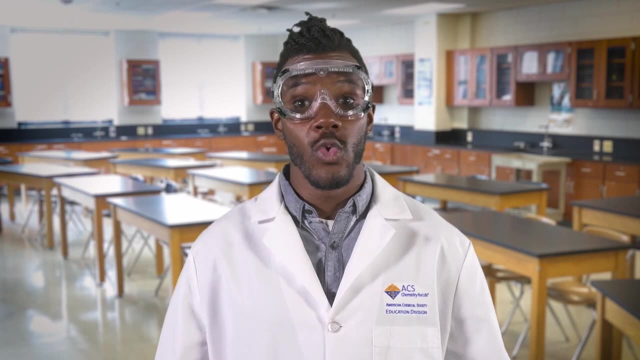 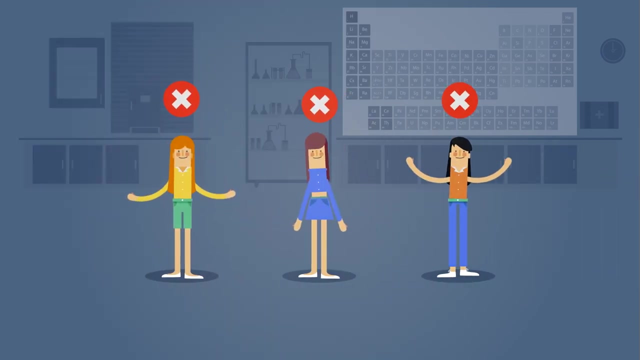 from exposure to chemicals. PPE is the most obvious way of preventing contact with chemicals, but it's not your first line of defense. Before you put on any PPE, you should think about how you're dressed for. lab Shorts, short skirts and t-shirts leave a lot of skin exposed. 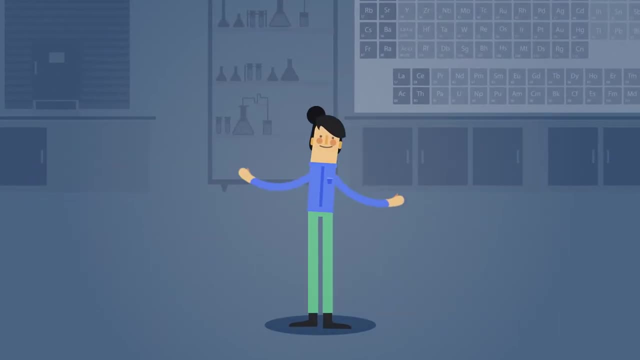 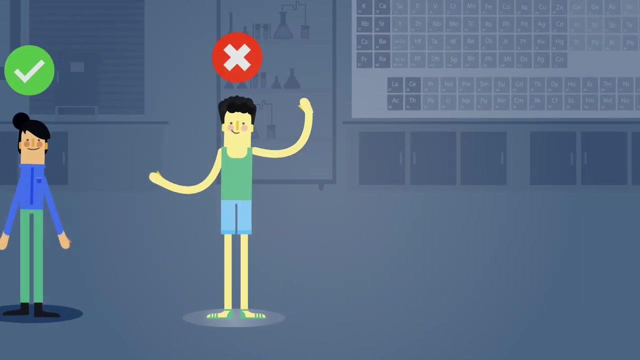 to potential spills. It's important to choose clothing that will protect your arms, your legs and midriff, And this goes for the guys too. You also want to avoid bulky and loose-fitting clothing. This could accidentally knock over equipment, get dragged through. 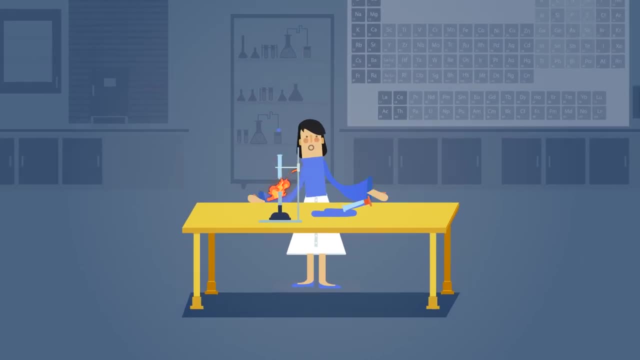 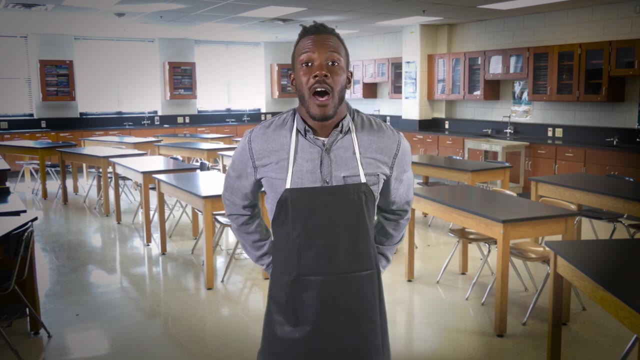 chemical spills or even catch fire if you're working with open flames. Your teacher may also require you to wear a lab coat or apron in the lab. Non-flammable, non-porous aprons offer the best and least expensive protection. But remember they work best when worn over. 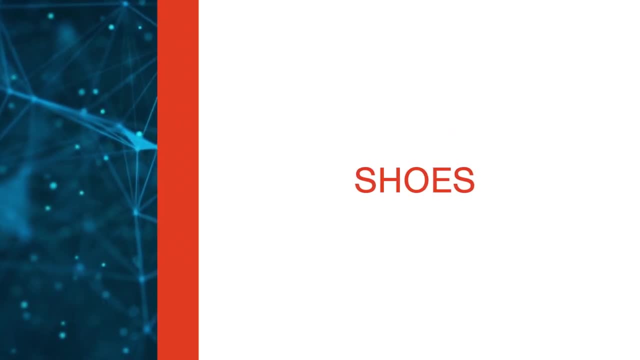 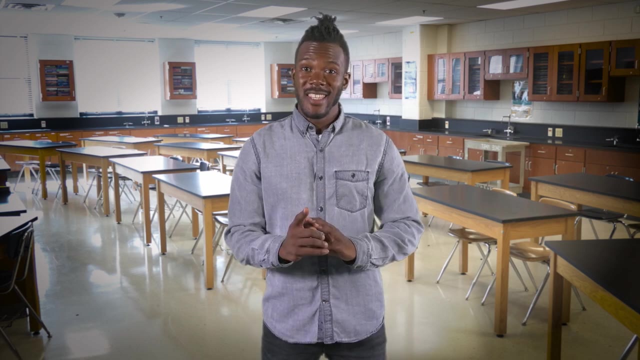 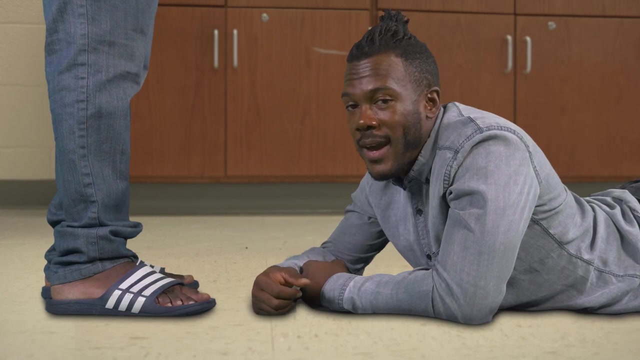 clothing that is appropriate for the lab. When choosing shoes for the lab, you should also think about potential spills and splashes. However, there's an added danger: Glassware or equipment could get dropped on your feet. For this reason, sandals, flip-flops and backless shoes are never allowed in the lab. 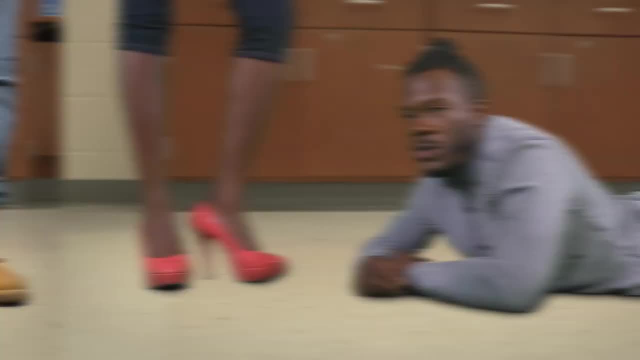 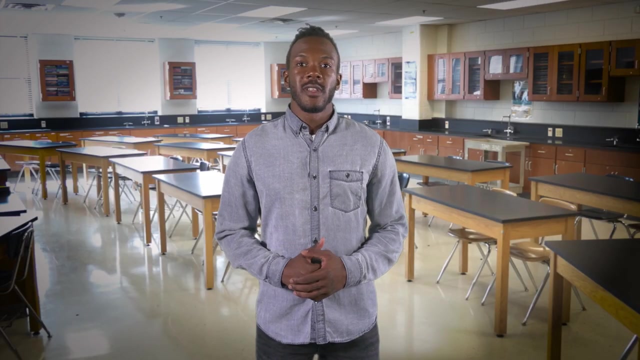 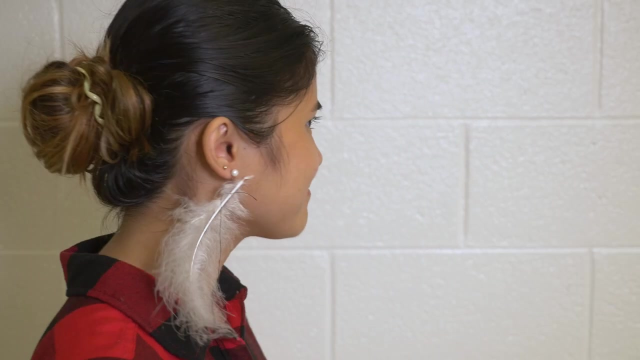 In fact, your shoes must completely cover your feet from heel to toe, which means no high heels or wedges. It's important to tie back long hair when you're working in the lab and to remove any dangling jewelry, such as earrings, necklaces or bracelets. Long.